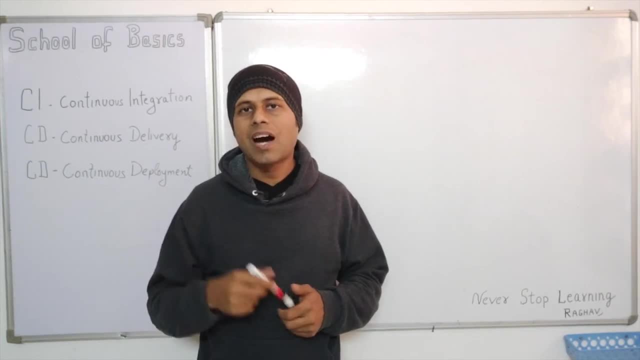 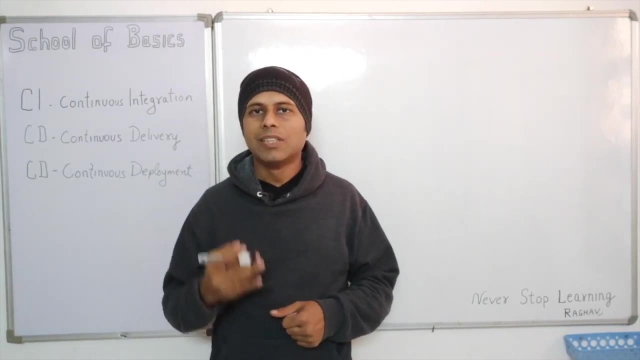 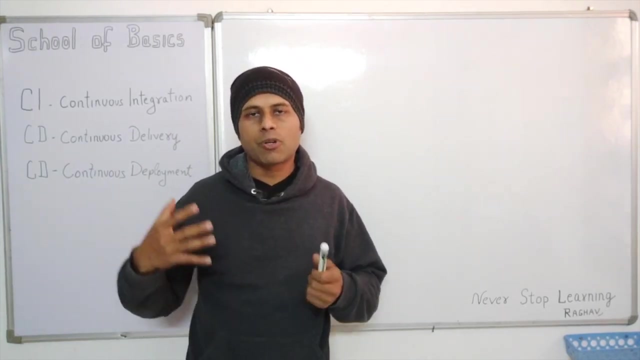 deployment. So let us see what exactly this is. and after this video, you can always explain CI CD to anyone with actual examples. So let's start- and I will start- with a real world scenario. in a project, in our organization, We have processes and it starts with a dev process. So any project, any 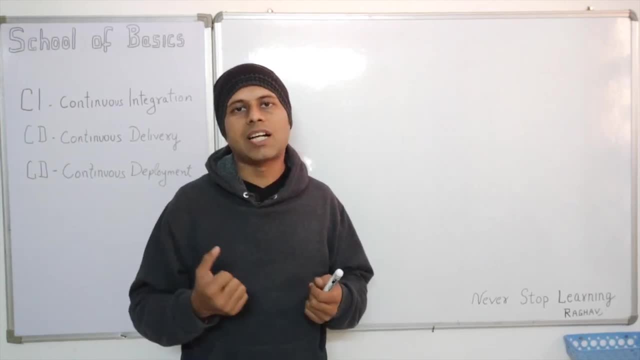 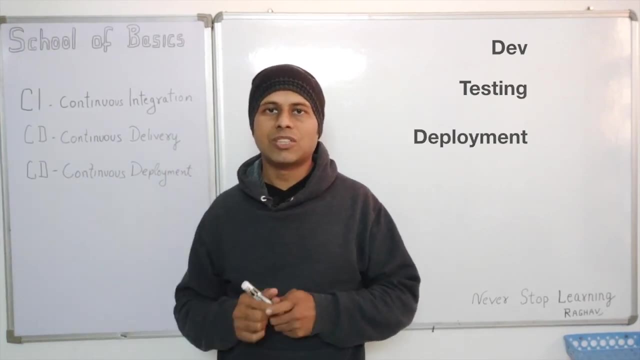 application or development. any software project starts with a dev process. So we have a dev phase, then we have a testing phase and then we have a deployment and release phase. So let me write down the phases. So we start with a development and release phase. 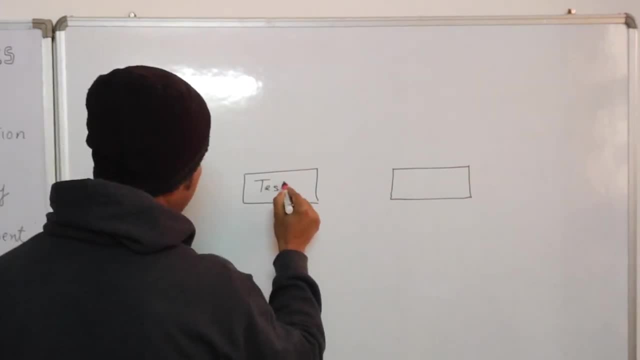 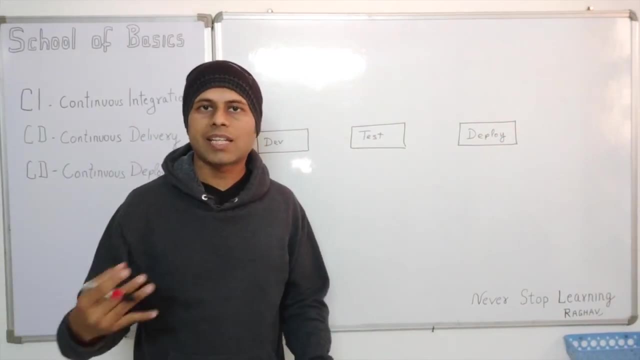 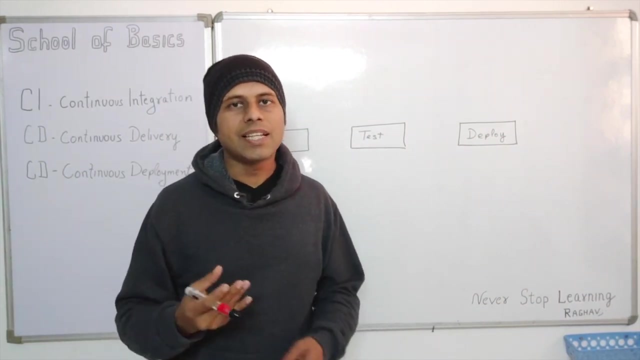 So we start with dev, then we have test, and then we have deployment phases and then we can have release, or release can be a part of deployment, or after deployment we do the release process. and I will tell you about that Now, coming to CI. CI stands for continuous integration and the CI process happens mostly into the. 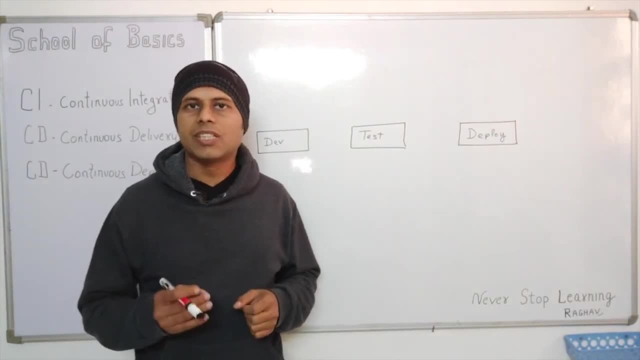 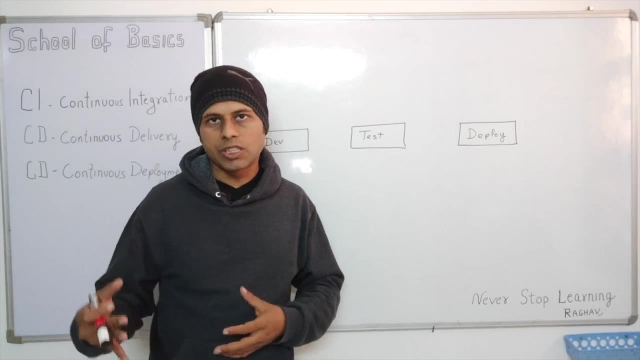 dev phase. Now, CI or continuous integration is the process where the team members integrate their code or their work in a shared repository, and this process is best achieved by using some SCM or source code management tool like Git, So they integrate their work on a daily basis. 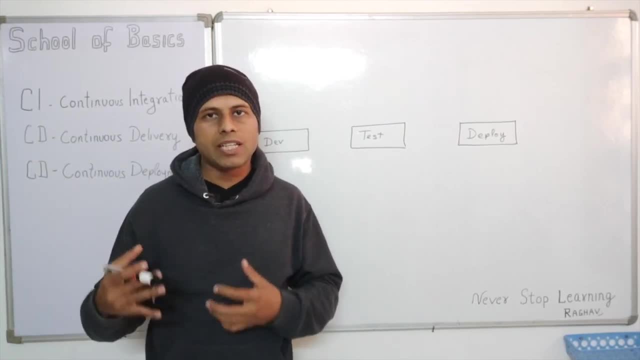 It is mostly done daily. That is once a day. everyone, everyone in the dev team, will integrteke and check in their work in the shared repository, and this check-in is then followed and validated by our automated, built and automated unit. here I am showing you on the fondog fairdev, where this technical 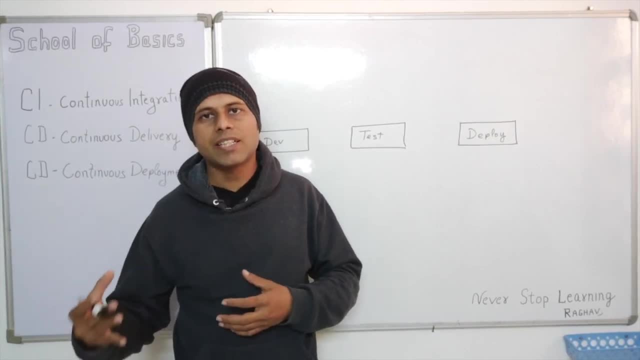 infrastructure is integrated into this shared repository very quickly and it involves a lot of things like technology, reading materials and a lot of other elements like software and vocab, and both these are fully integrated into the shared repository. So let us start this documentary session. It starts with a. 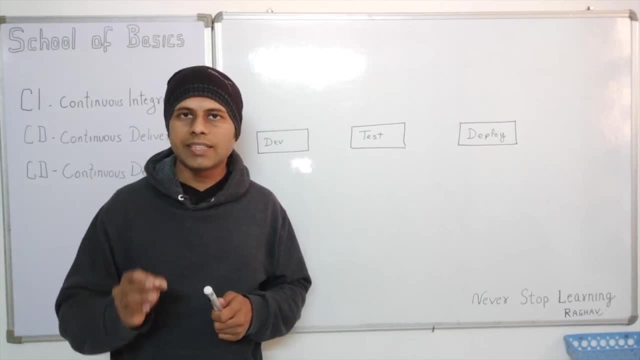 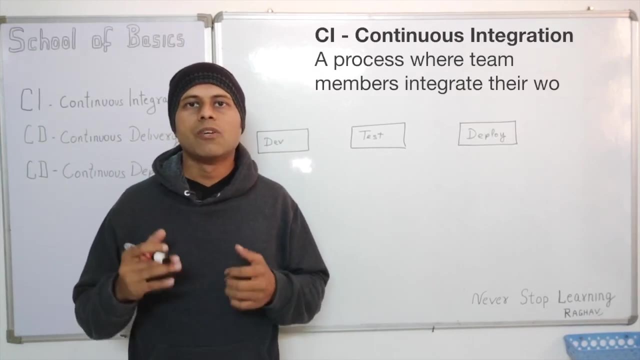 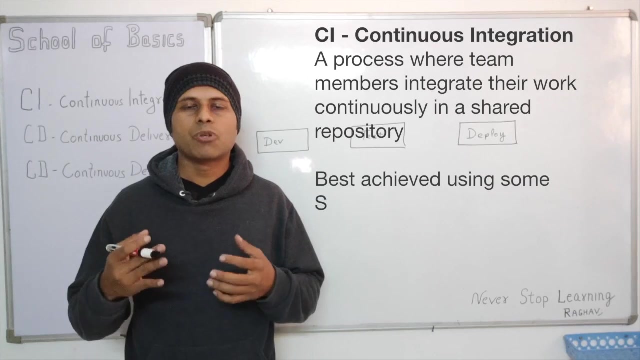 automated unit tests. so this is what the ci process is, and you can also see the definition on your screen. so let me again repeat: ci or continuous integration is the process where the team members integrate their code or their work in a shared repository. this process is best. 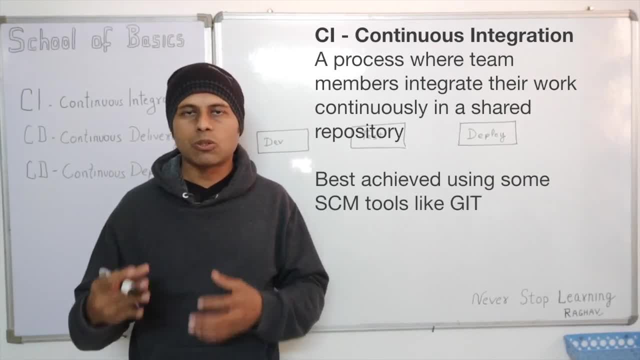 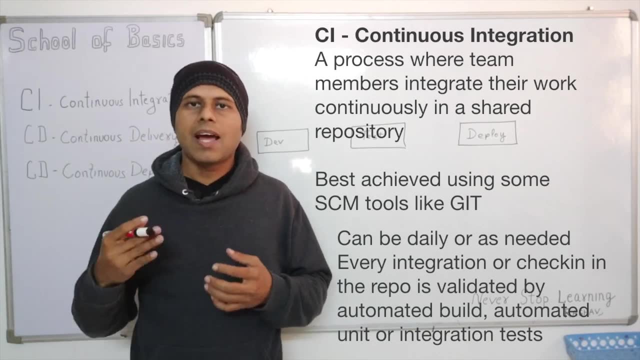 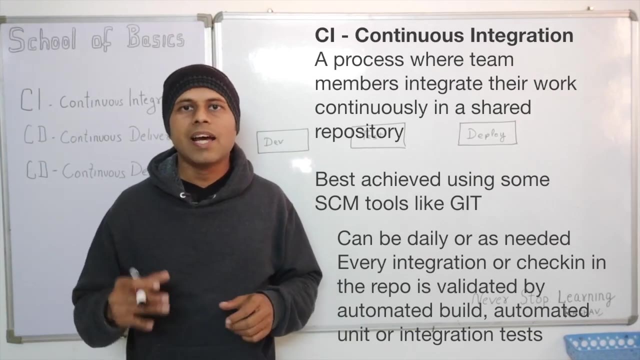 achieved using a scm or source code management tool like git, and every check-in is followed and validated by an automated build and automated unit tests, and there can also be some automated integration test that we run to make sure that everything is fine, there are no errors, and this 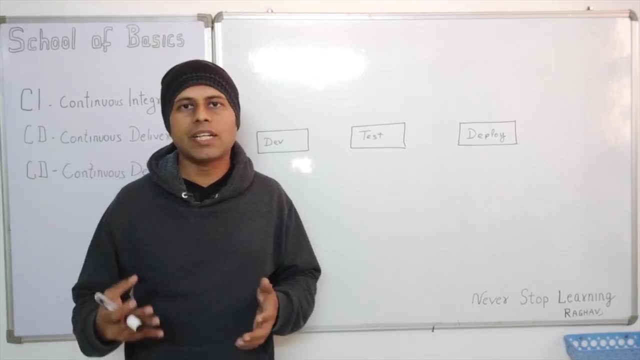 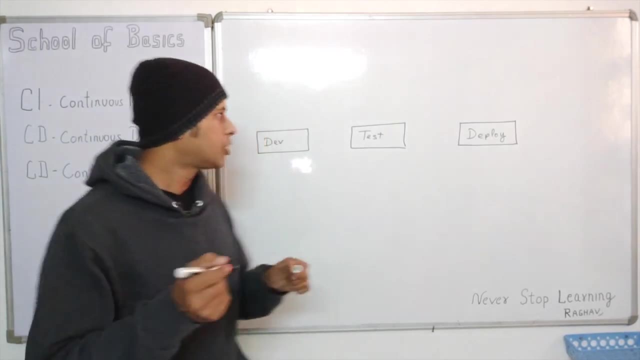 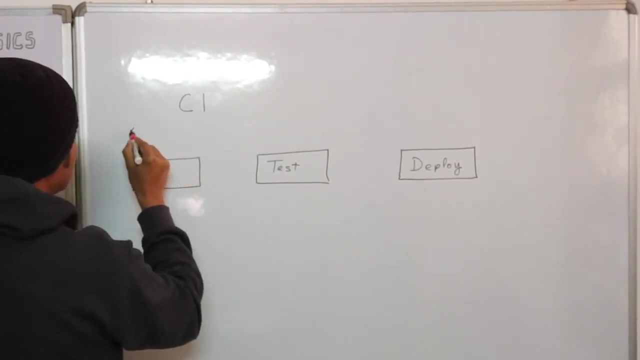 process is mostly done daily. that is, once a day, but as per your need, as per the requirement of the project, it can be done as frequent as needed. this is the process of ci, so ci process, so the ci process. so the ci process, so the ci process. 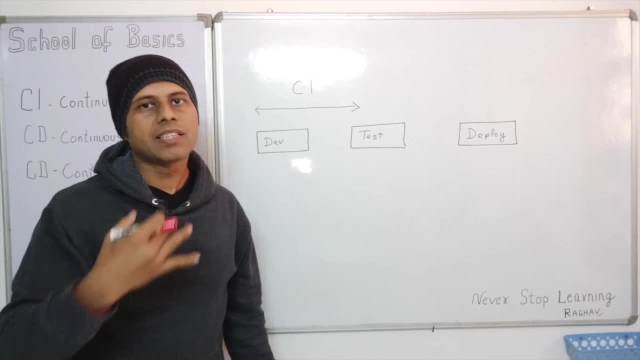 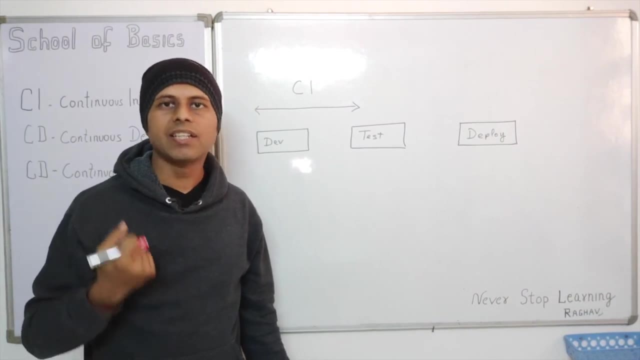 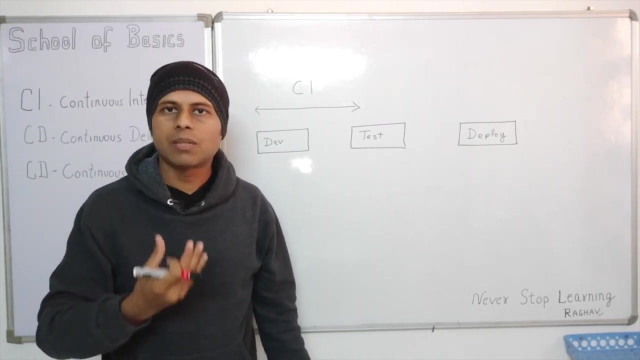 is expands from the dev phase until some part of the testing or the qa phase, because most of the tests are unit tests which are automated at the dev end and they are they run automatically after the build or after there is an automated build, but then we can also add some of the 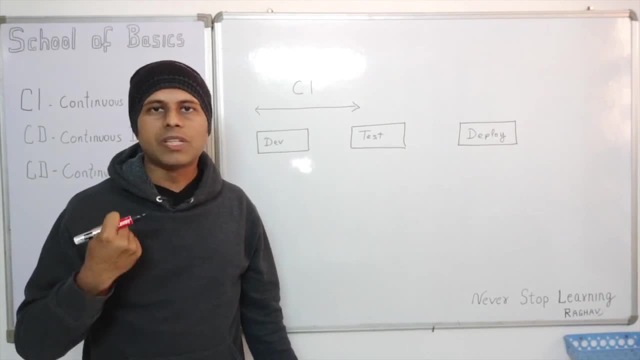 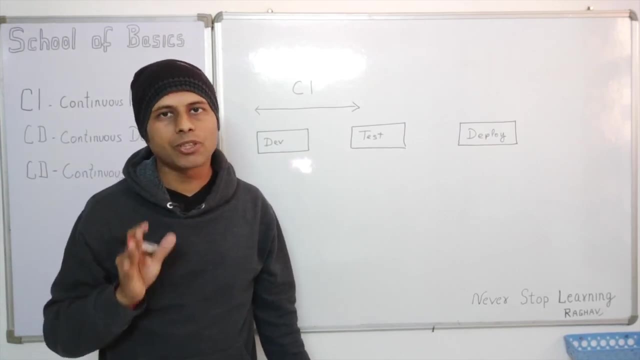 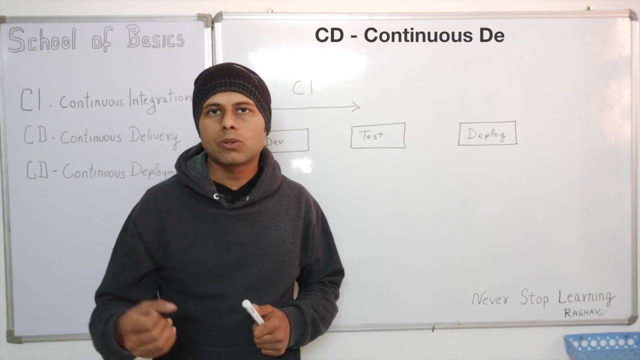 integration tests from the test environment and then we can say that the code we have deployed today or the code we have integrated today is all fine without any errors. so this is the process of ci now coming to cd or continuous delivery now after the ci process. if we also do a deployment, 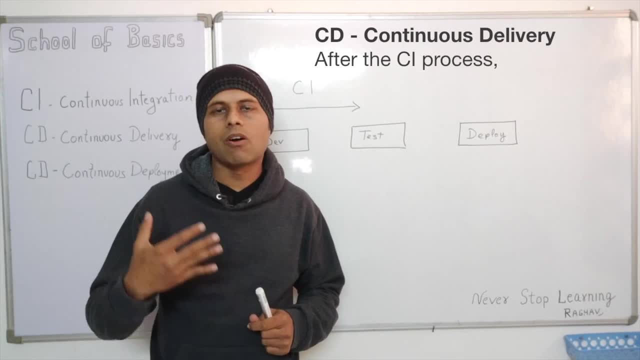 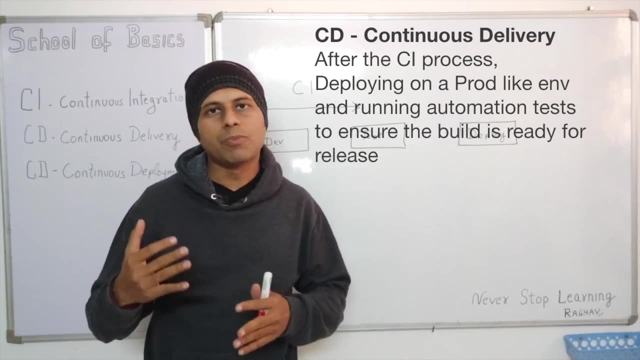 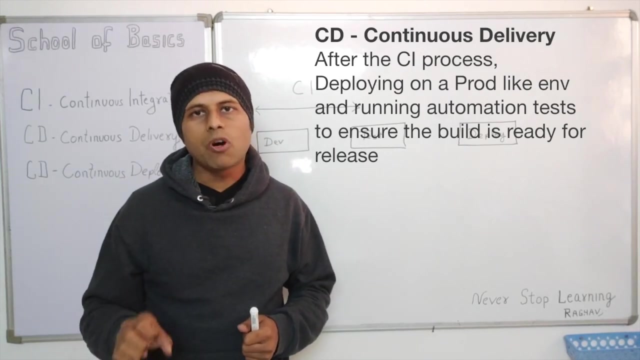 on a production like environment- it can be a qa or can be a staging environment- and then we run some automated tests to ensure that this code, this build, is now ready to be deployed. we call this process as continuous delivery. so basically, the goal or the aim of continuous delivery process is: 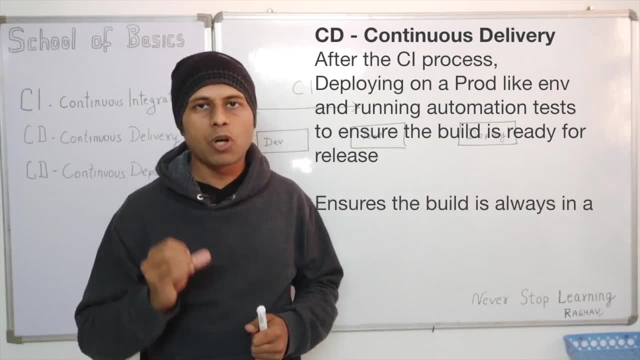 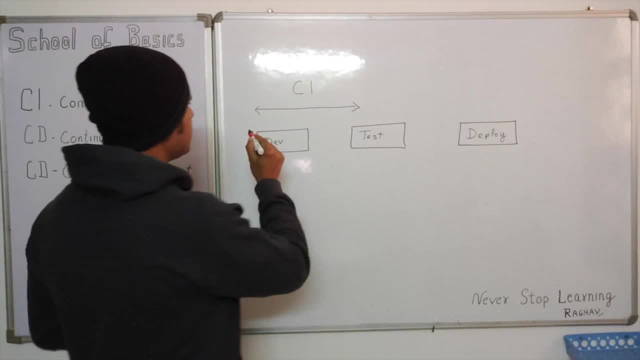 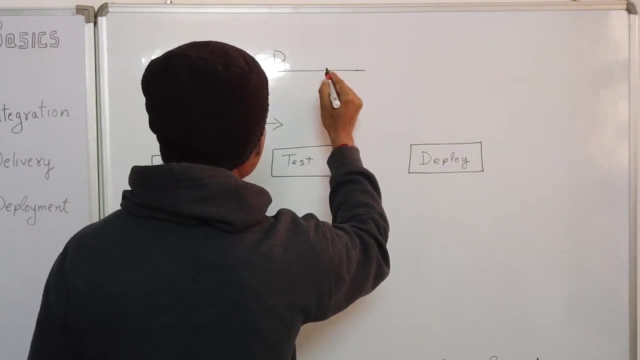 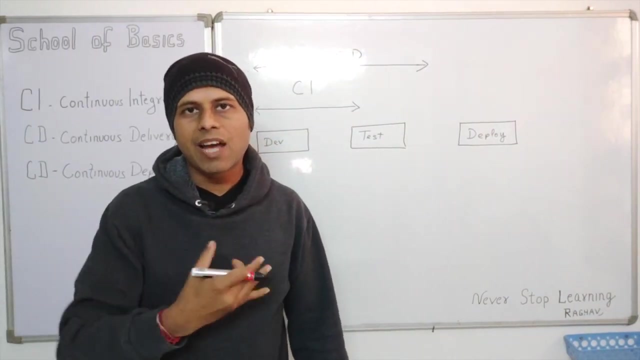 so basically, the goal or the aim of continuous delivery process is to make sure that the build is always in a deployable state or a deployment ready state. so continuous delivery, or cd, expands from dev until the testing phase or the qa phase, and, if i also include the environments. 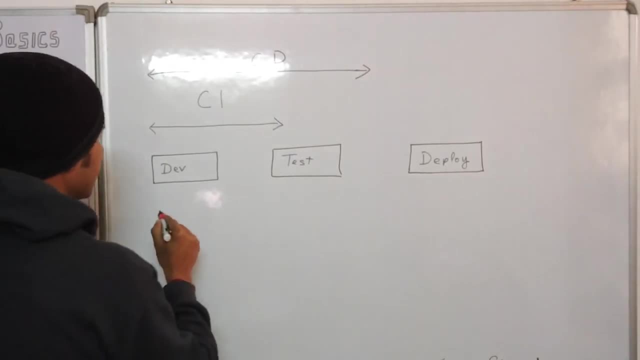 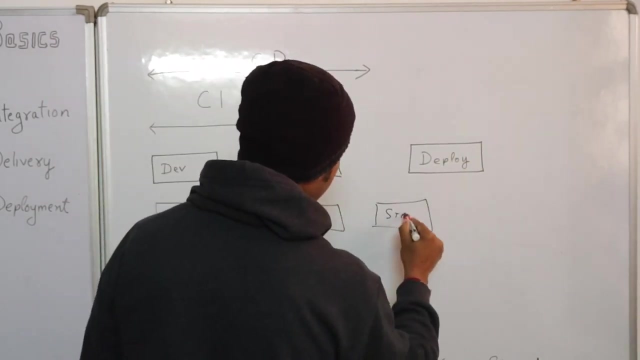 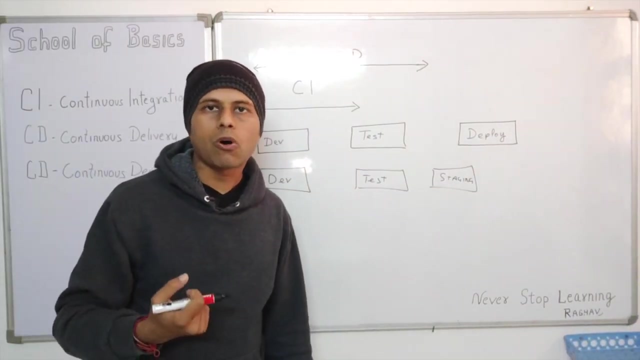 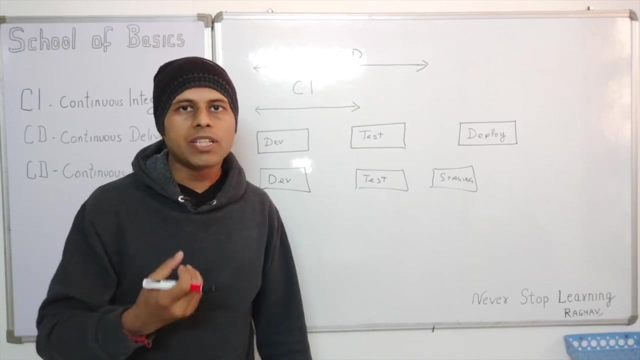 here to make it even more clear. so we have a dev environment, we have a test environment, we have staging. now, staging environment is a production-like environment. it is sometimes also called as pre-prod environment or pre-production environment, and the goal here is that we create a environment or we keep our environment, exactly like a copy of our production. 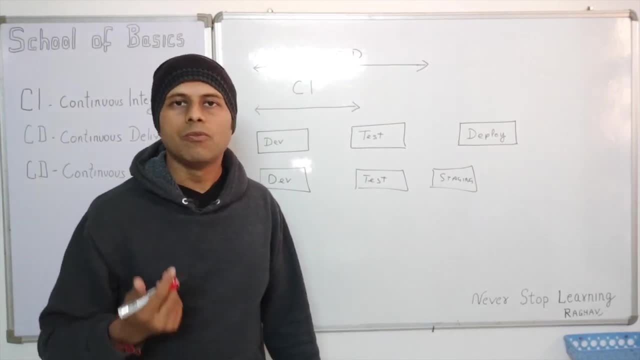 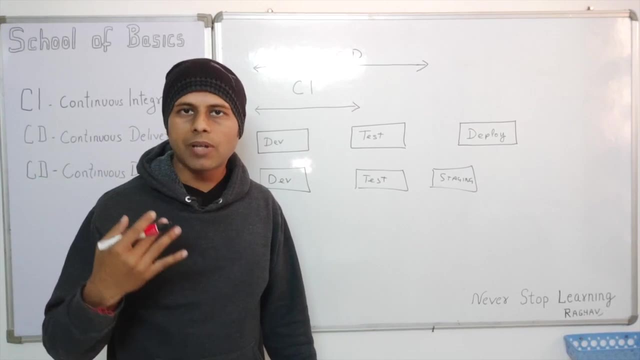 so that before deploying anything on the production, we can check it on the pre-prod or the staging environment. and also, if we want to check anything, instead of going to the actual prod environment, we can check it on the staging or the pre-prod environment. so 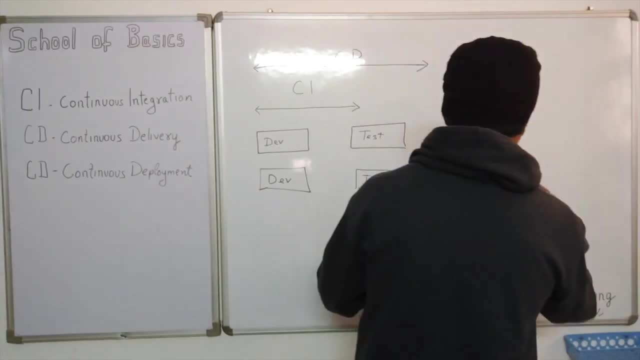 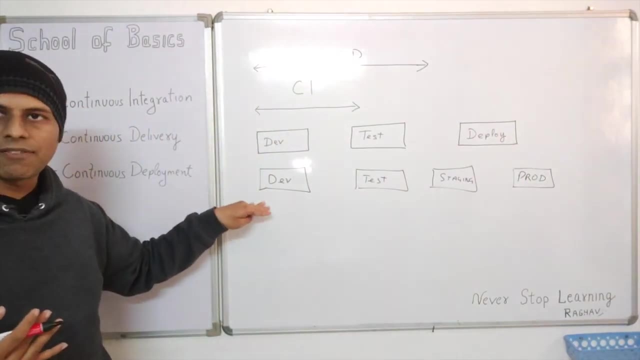 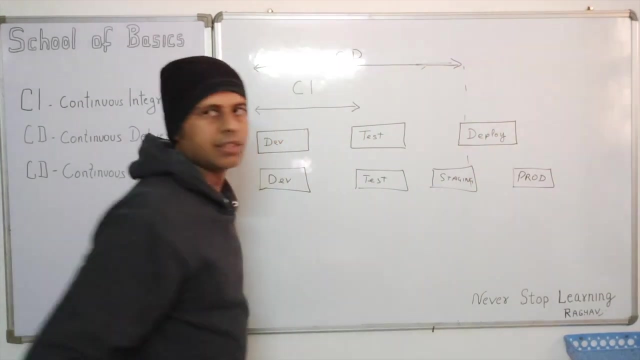 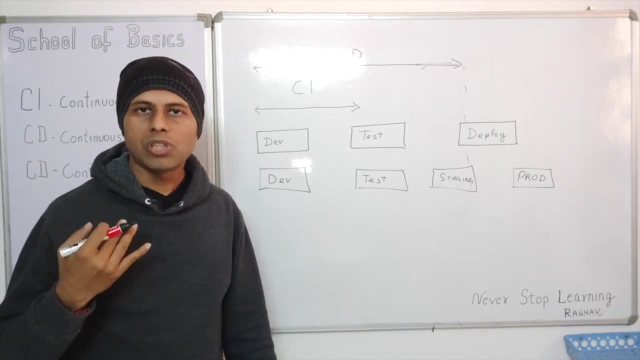 we have a staging or pre-prod here and then we have a production environment. so if i talk about a continuous delivery, it starts at the dev environment and then goes until the staging environment. so it will go until here, which is the staging environment. so here the goal is that our build, our code, is now ready to be deployed on any environment. so this is 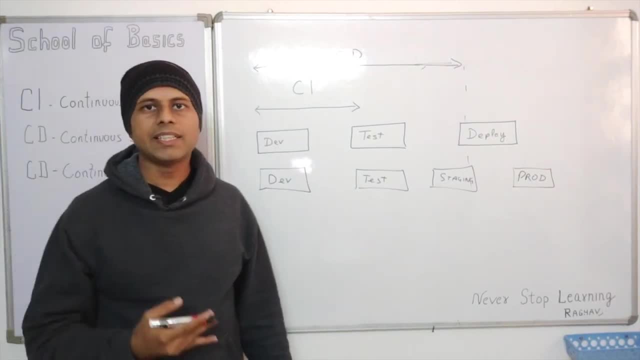 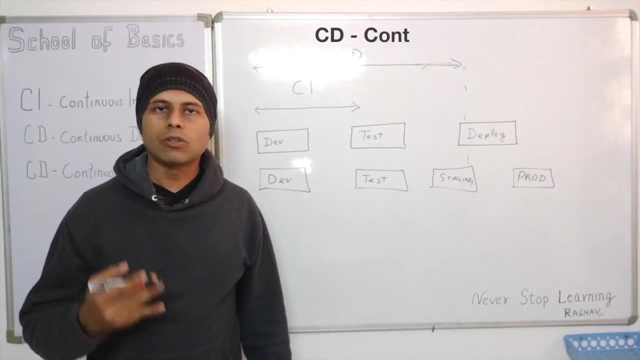 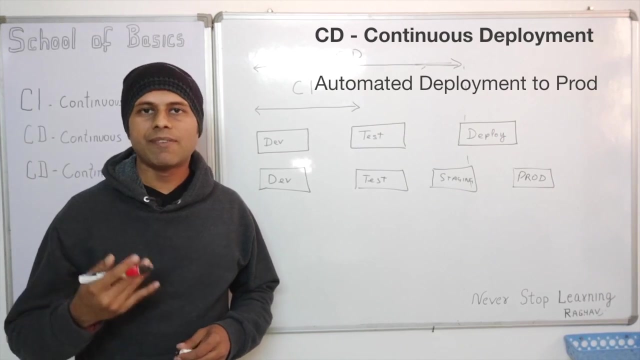 continuous delivery. now, when we talk about the next cd, that is the continuous deployment. here we, along with doing cie and continuous delivery, we also do a production deployment. so this is automated deployment to production, and every change, every release that passes through all the automated tests is then directly delivered to this cd and that is where it is used for the 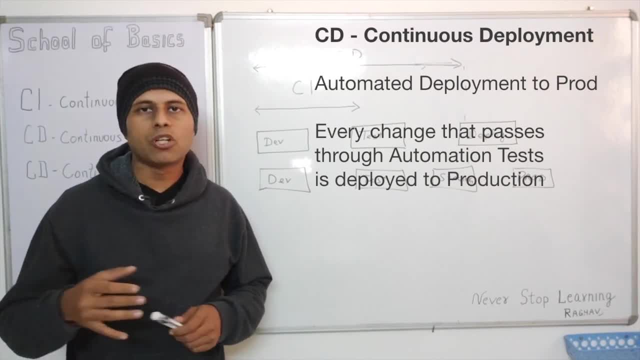 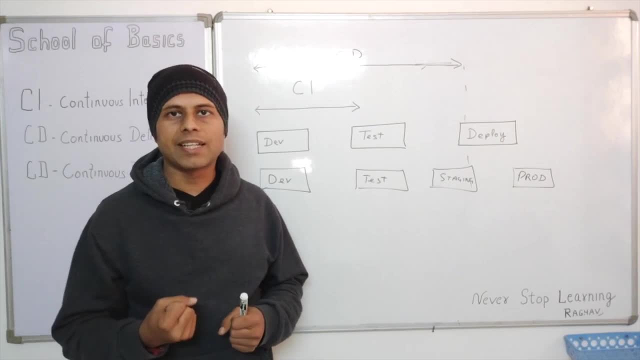 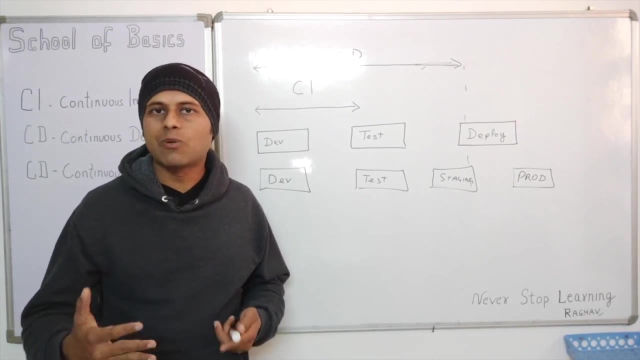 production deployment so there is no block to the production and also for the production deployment deployed to production environment. now this may not be practical in some of the organizations that they do not have so frequent and so short release cycle, so continuous deployment is not done automatically. but then there are organizations who do very frequent and very fast deployments if 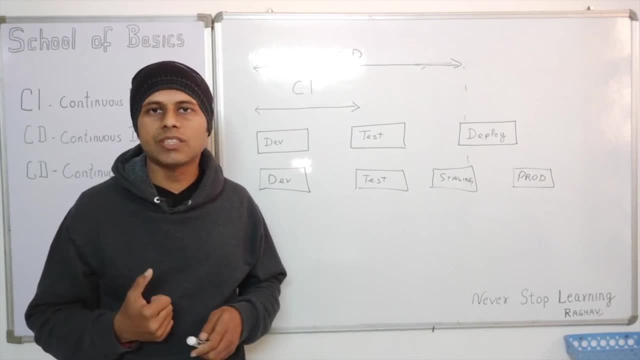 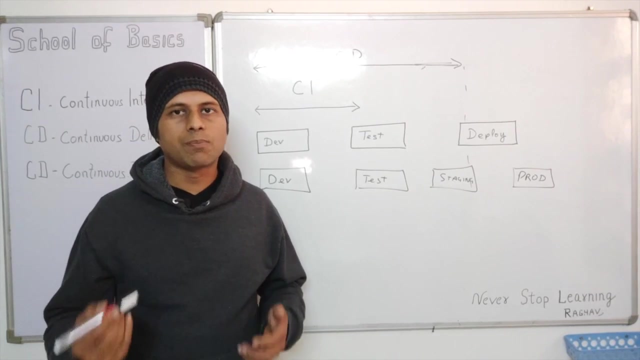 you think about facebook or other very big organizations where we do some changes on a basis. there we follow continuous deployment, because every change that passes through all the stages, all the automation tests, is then directly deployed into production. so this is continuous deployment. so along with CI, CD, we are deploying to production, which is again a 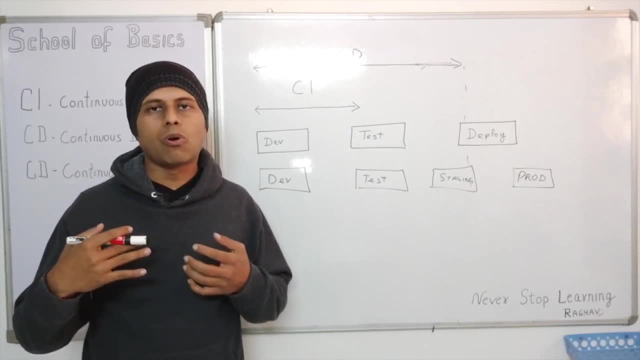 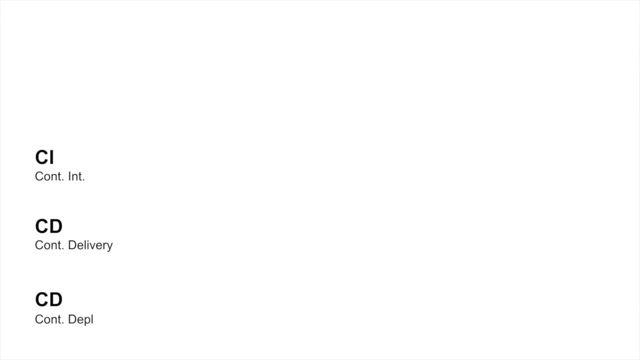 automated process and all the changes that passes through, all the automated tests are deployed directly into production. let us now understand CI and CD in a very, very basic ways. let us now understand CI and CD in a very, very basic ways in terms of the stages and the environment. So let us suppose we have these three very 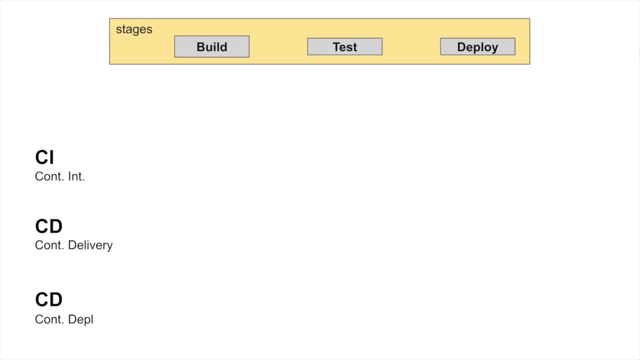 basic, typical stages. in any project, that is, build, test and deploy. We also have a release stage, But for now let us look at these three basic stages. When we talk about CI or continuous integration, then CI expands from the build stage until some part of the testing stage. 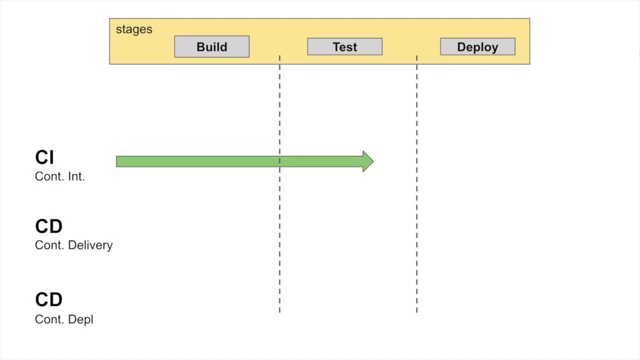 because here we are doing the integration of the code And then, after a successful build and code integration, we also run some unit tests within the dev environment and can also run some functional tests from the QA environment to make sure that our integration, the integrated code, is now working and there are no errors or no issues. So CI expands from the build. 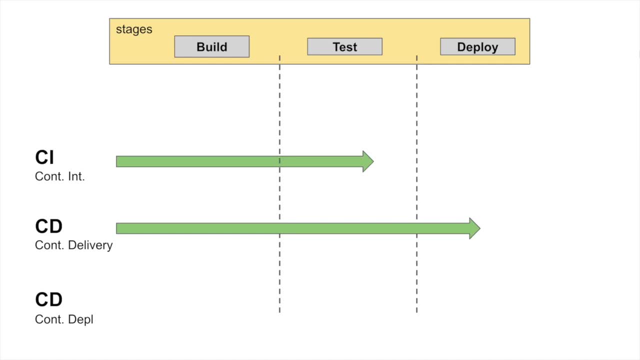 to some part of the test stage. If I talk about CD, that is continuous delivery, it includes the CI process, and then we also deploy it on a pre prod or a staging environment. So here the continuous delivery process will expand until the deployment stage. And now 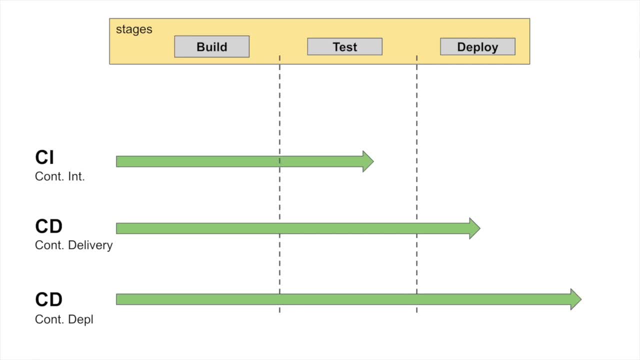 when we talk about continuous deployment in CD or continuous deployment we do CI and CD. that is continuous delivery. Plus we also do deployment on the actual production environment. So here we can say that we are also doing the release of our software to the final production environment. So CD or continuous deployment process will expand until the release stage. 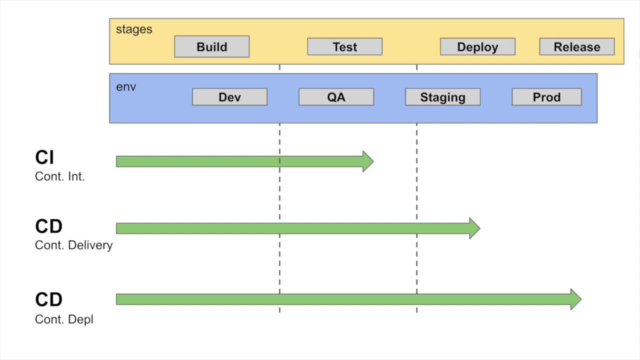 Now, if I also include the environments, that is, the dev environment, the QA, the staging and the production environment, Now the CI process will expand until the QA environment. The CD or the continuous delivery process will extend until the pre production or the staging environment, And then the continuous deployment process will extend until the final. 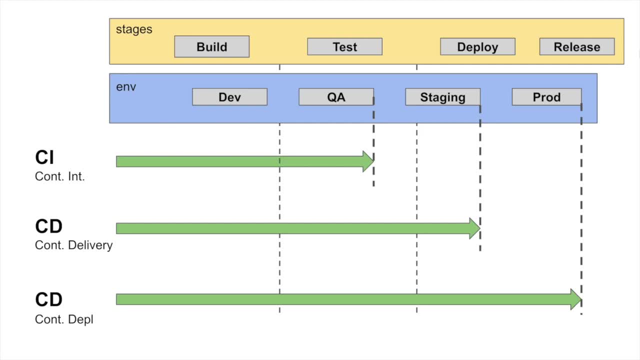 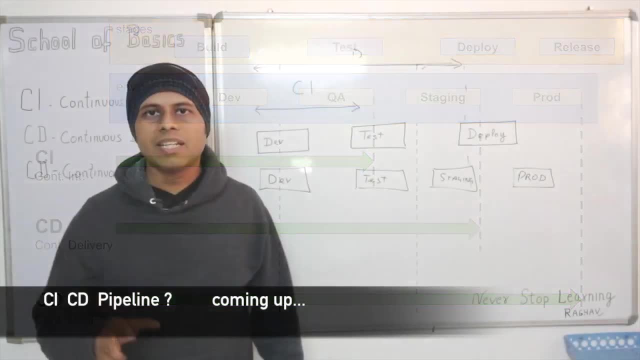 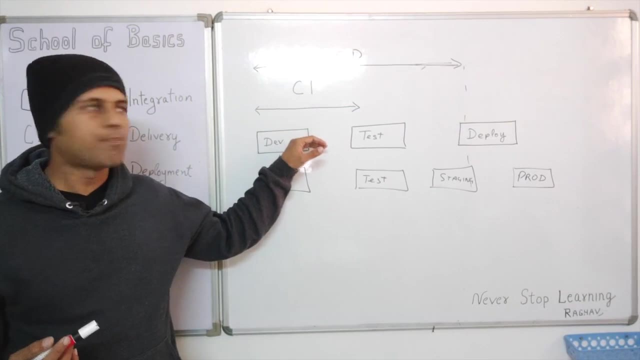 production environment. So this is, in the very, very basic ways, This chart. you can keep it in your minds forever And this is the complete process of CI and CD. So again, if you see the phases, CI is mostly in the dev phase and can also expand until some part of the testing or the QA phase. CD. 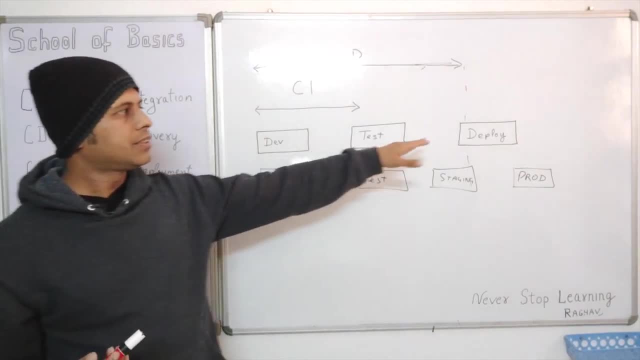 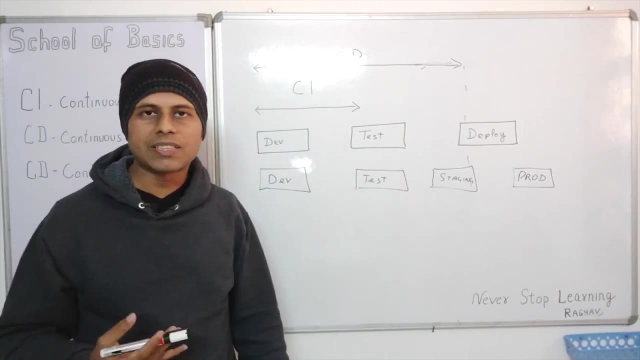 is from the dev phase, It is CI plus the deployment to a staging environment so that we can run some our automated test cases. The integration, the acceptance, the deployment, the deployment, the deployment, These are all the automated test cases, all the automated functional test cases. And then